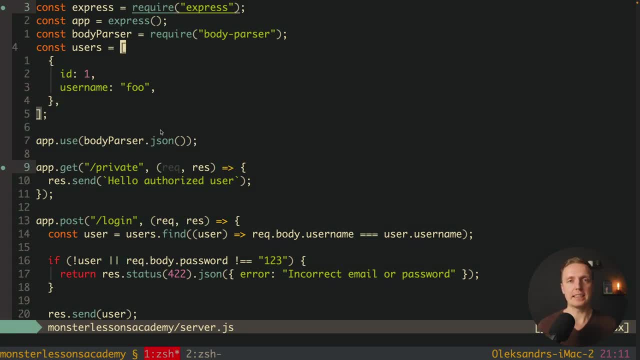 and I created here an array of users. The main idea is that I won't show it with the real database. we will simply store all our data inside memory of our node process, And this is totally fine, because it doesn't really make any difference if your user and 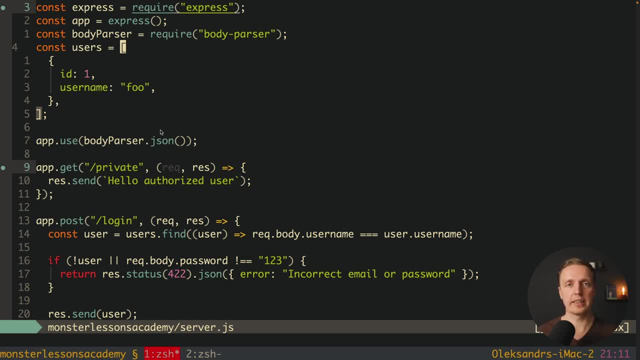 your session is coming from the database or just from the array inside your memory. It is working in exactly the same way. As you can see, here we have two different requests. First of all, app, get on slash private, and here we simply sending back a string. 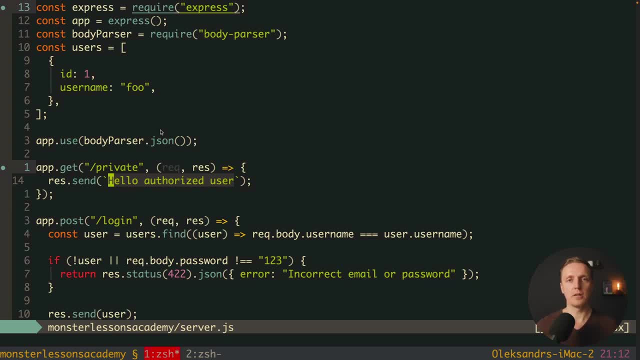 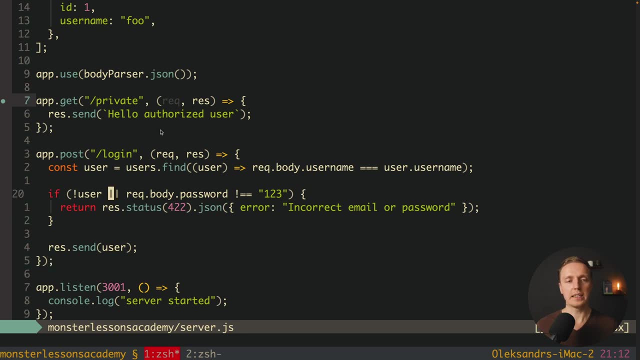 The main idea is that we want to make this request only for logged in users. This is why here we must update it later. And also here I have a login request where inside we are trying to find a user by body user name, Which actually means inside our body to login. 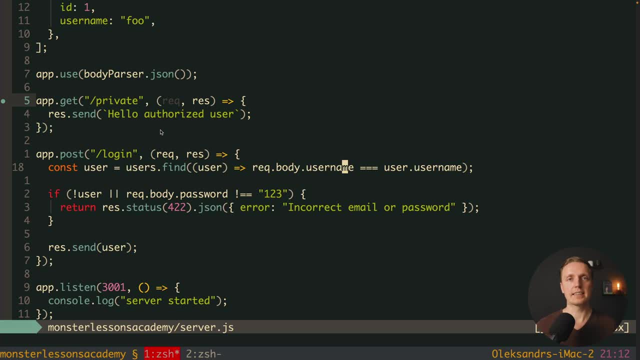 We are providing user name. We are providing user name, We are providing user name and password, And this is a typical authentication inside any project. The main difference is this single liner. inside real project will be a database request, But in our case here we are just trying to find a user inside our array of users by unique. 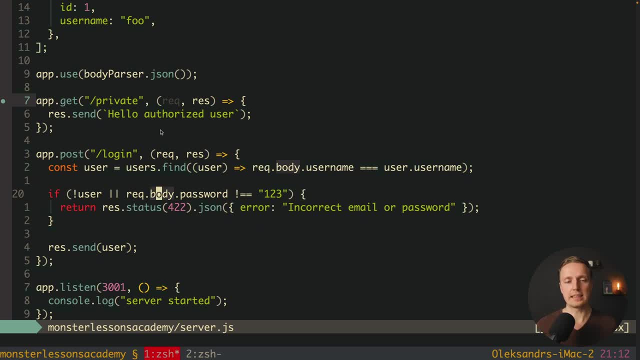 user name. If we didn't find a user or our password inside body is not 123, then we are throwing an error. If everything is fine, then we simply return a user And inside real application you won't have a password 123.. You need to implement password comparison. 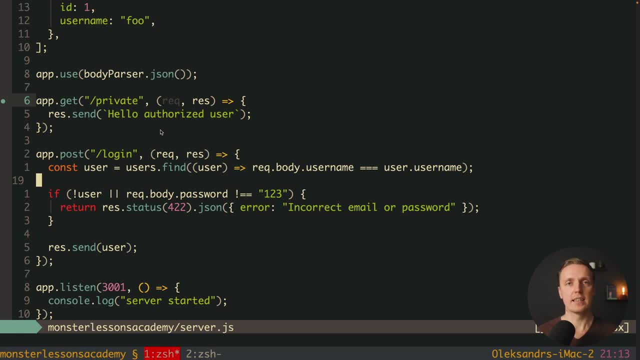 But it doesn't have anything to do with cookie authentication. This is why I don't want to make this video more difficult by using real database. Let's check how our application is working. As you can see, our server here is started. We can jump directly to postman. 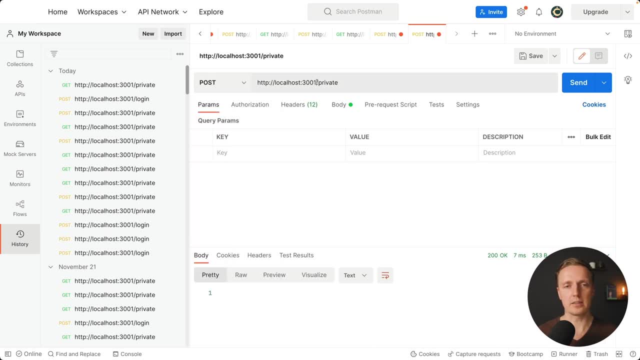 And here we want to make a post request on localhost 3001 slash and here we will be logging And inside our body, we must provide user name and password And, as you can see, as a result, we are getting our user with id 1 and username fum. 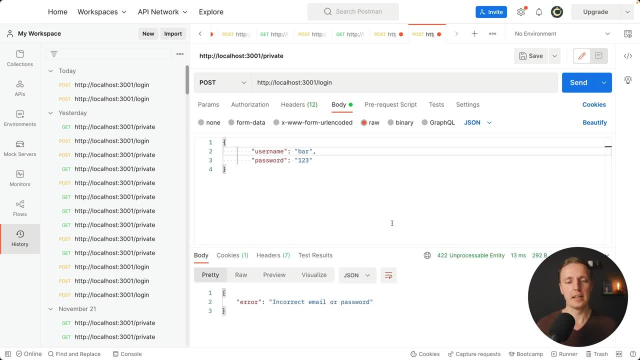 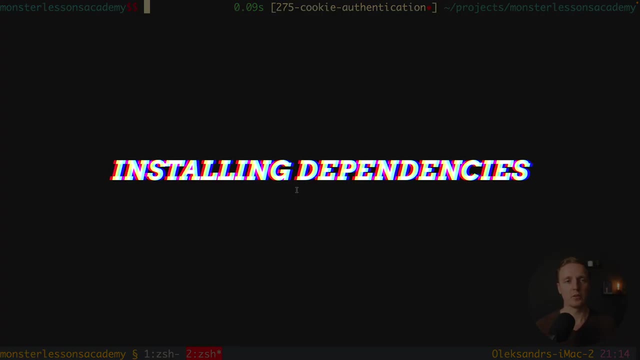 Obviously, if here I will provide a user which does not exist, we will get incorrect email or password, Which means it is working exactly like a real application. Now we can start to implement cookie authentication on top of it, And actually for this we must install two additional packages. 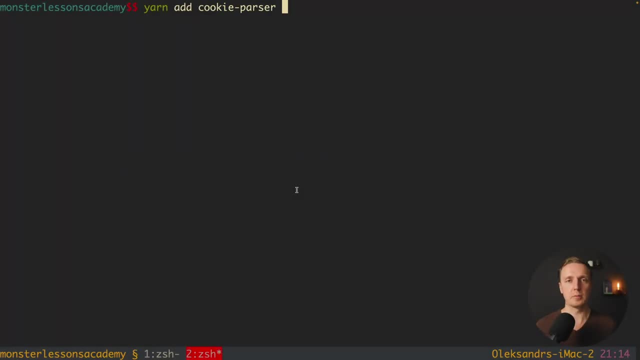 So here we can write yarn add, and first of all, it is cookie parser, because we are using express on the backend, And cookie parser package helps us to work with cookies in an easy way. And the next package that we need is uuid. This is a special package which allow us to generate unique strings. 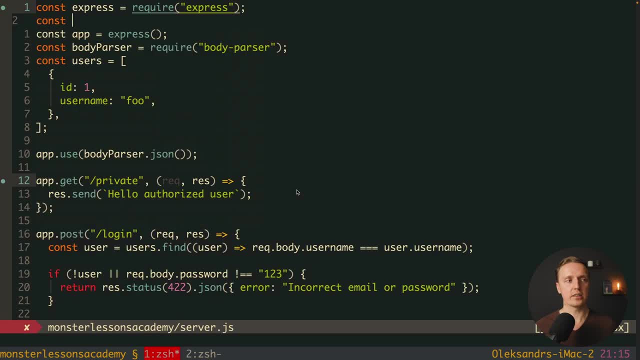 Now let's jump inside our project, And here on the top, we can require first of all, our cookie parser, And here it is, coming from our package that we just installed. This is cookie parser. Now, here, after our body parser, we can add cookie parser. 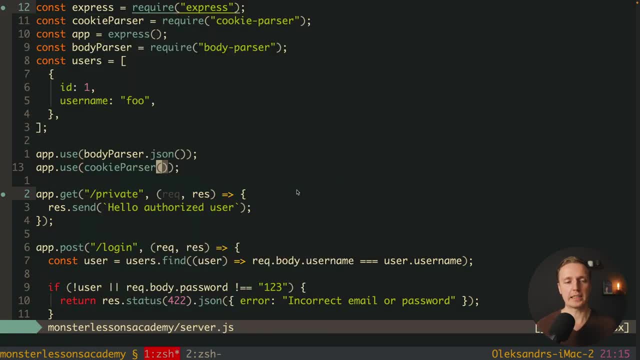 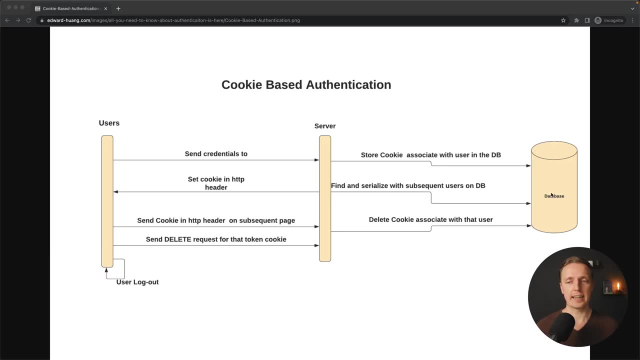 This is why here app, use cookie parser, Just with round brackets, and we are good to go. The next thing that I want to create is a storage for our sessions, And actually from this diagram you can understand that inside our database we typically will have an additional table with all our sessions. 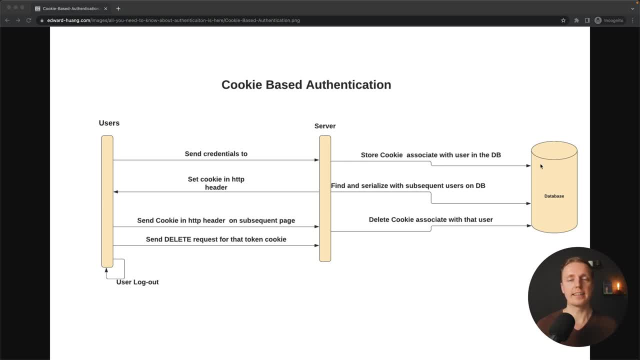 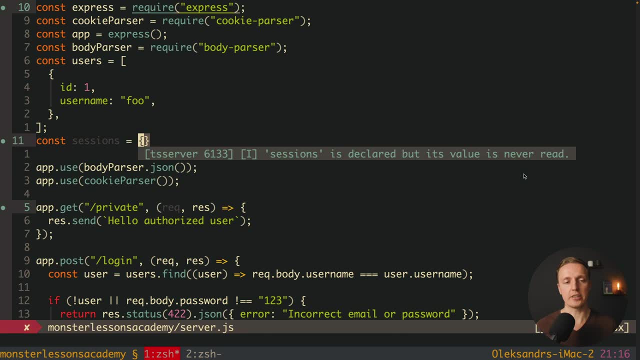 And every single time when the user is logged in, we are storing this new session inside the database. In our case, we have our database here and this is just an object with our sessions, And every single time when we are logging in a user, We are storing new session inside our sessions. object: 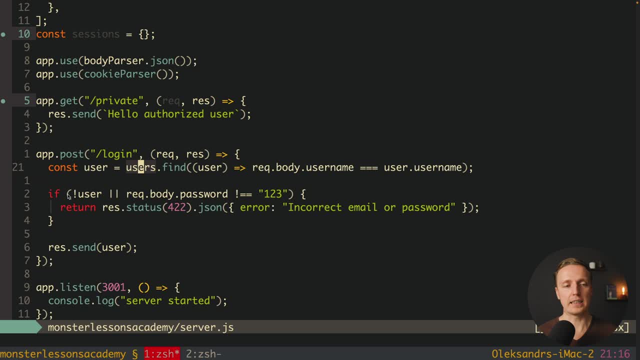 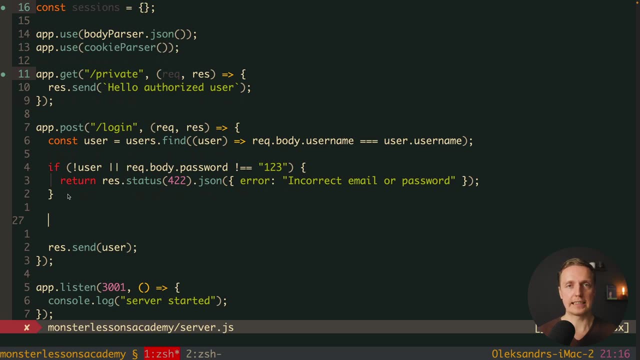 Now we need to update our login method. This is totally fine to get here a user and check if it is a valid user, But after this we must generate this unique string, which will be our cookie header and which we will store inside our sessions. 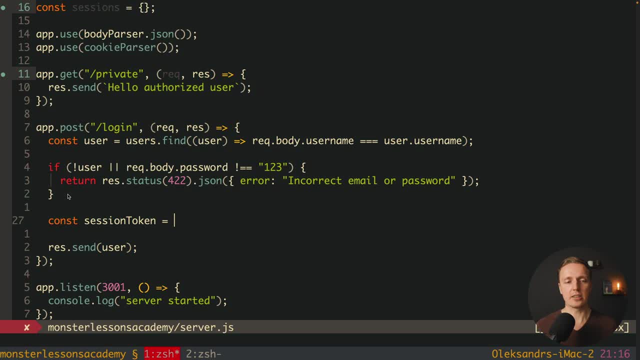 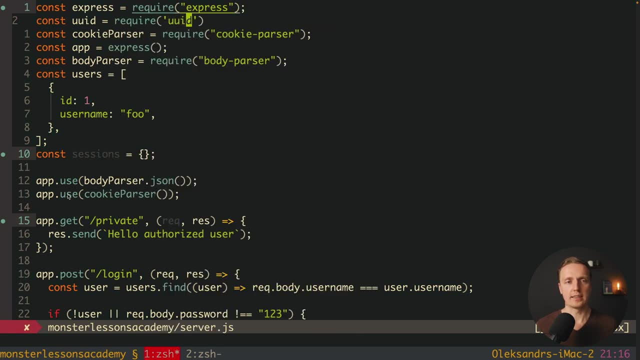 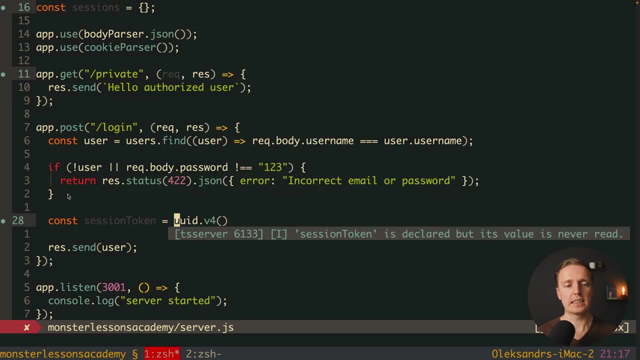 This is why here let's create our session token, And session token is just a unique string. This is why here we can require a library uuid That we just installed. Now, here inside our session token, we can simply use uuidversion4.. And it will give us back a unique string. 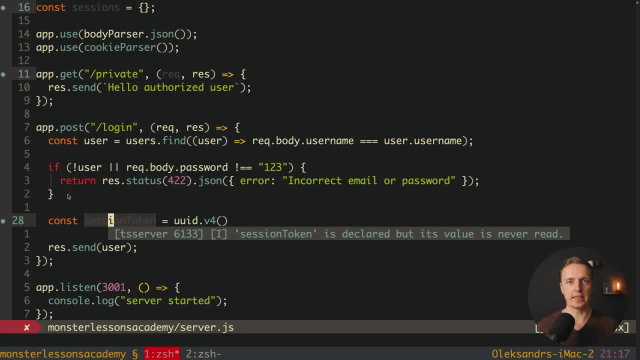 The next thing that we want to do is generate our expiration date. The main idea is that we want our cookie to expire. If, for example, you are working with money and you are implementing banking system, Then maybe you want an expiration time like 5 minutes. 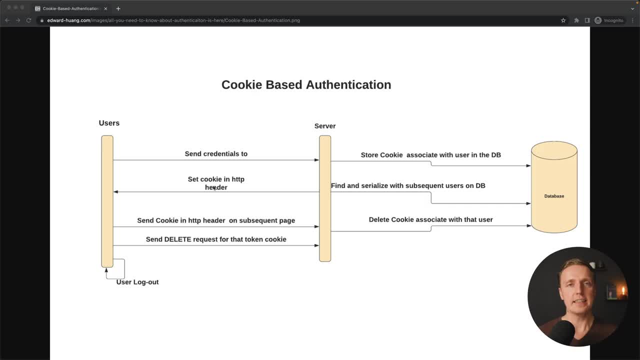 Because your application must be really safe. The idea is that when our cookie is expired, it will be simply removed from our client And we should not do anything about it. Now we want to create our expiration date Because we don't want our cookie to last forever. 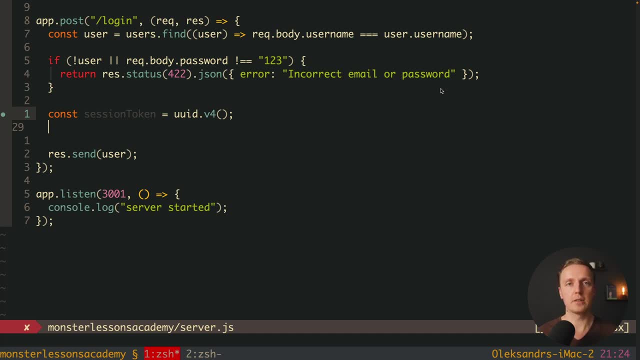 At some point we want to log user out. If you are working, for example, in banking system, Then it make a lot of sense to make a short expiration time. If it is not that important, Then you may set your logged in time for one year, for example. 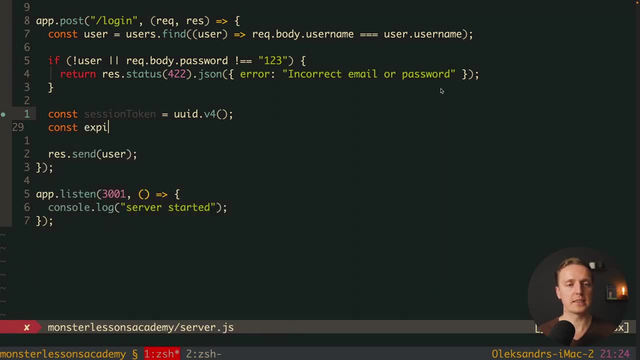 This is why here we want to create A new property which will be expires at, And here we can simply call new date, And this is a current time Set, full year- And inside we want to provide exactly the same date Plus 1.. 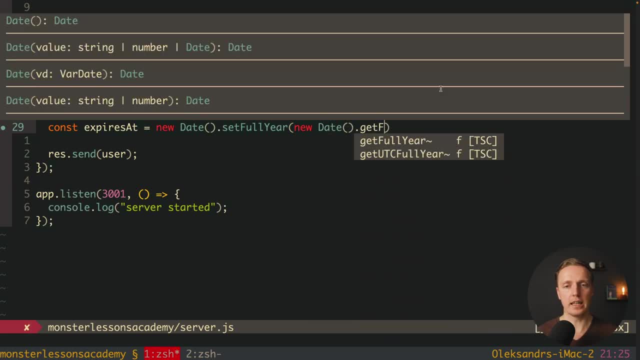 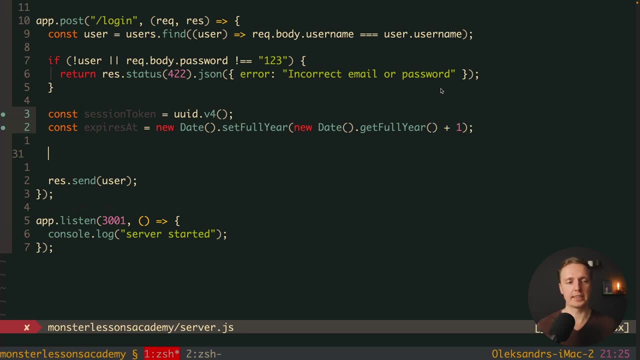 This is why here, new dategetfullyear plus 1.. Now we want to store our session inside the database, And our database is the object sessions. This is why here, inside our session object, we can write session token. This is our unique string. 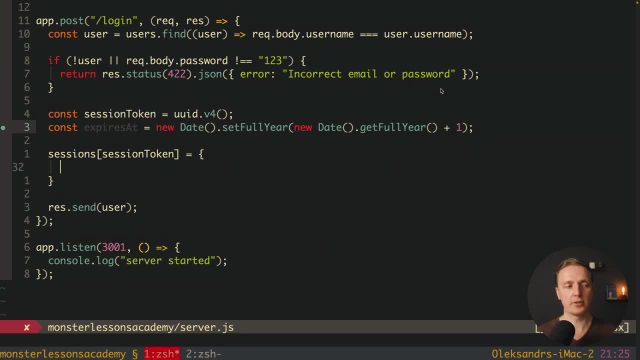 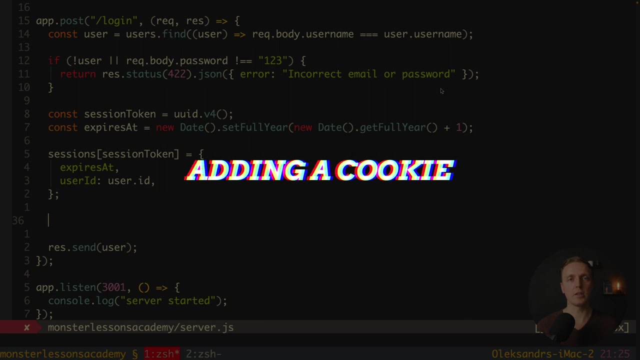 Of our session And inside we are writing the object, First of all with expires at And secondly with user id, Because this is exactly our user that we want to get later from session And find it inside database. So we successfully stored our session. 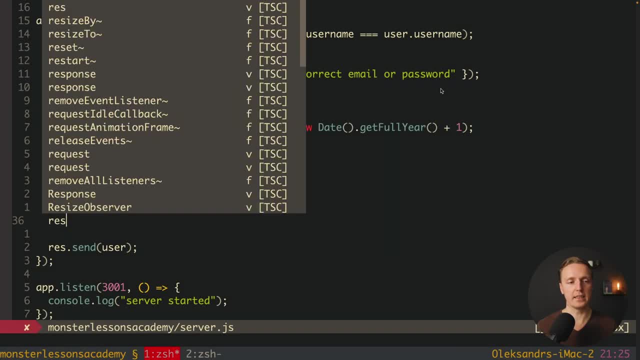 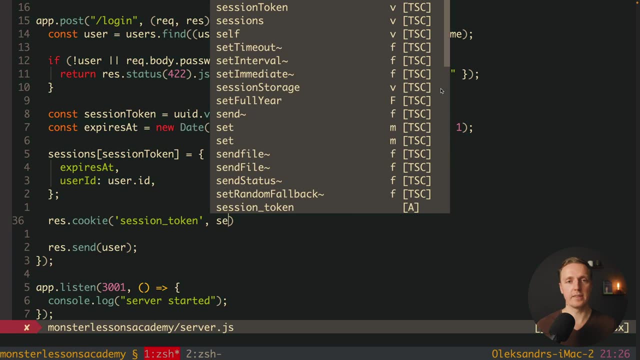 Now we must add a cookie to our request. This is why here, res cookie, And we are setting here first of all some name, For example session token. After this we are setting a value. This is our unique session token, And the last thing here will be our options. 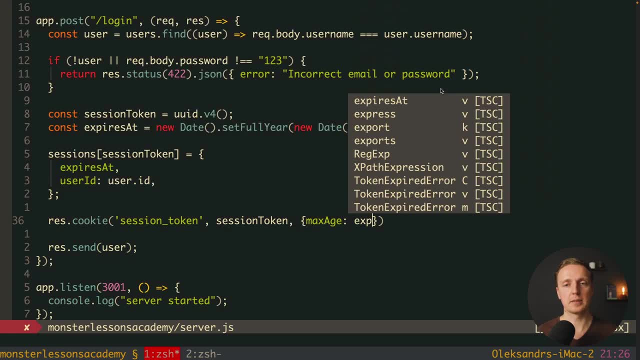 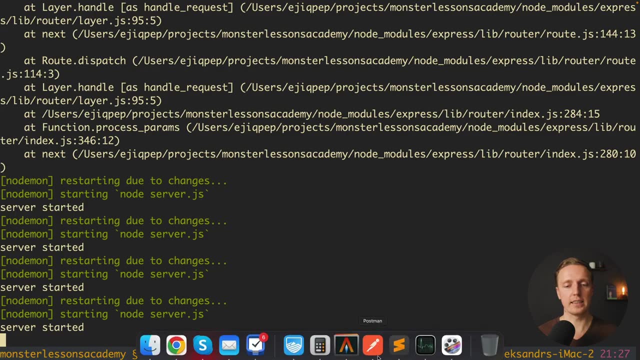 And we want to set here max age Which will be our expires at. This is exactly when our cookie will be removed. Let's check if it's working. I don't have any errors here. Let's jump inside postman and hit send. 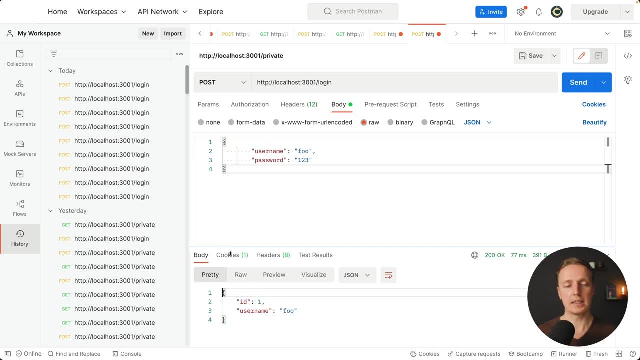 As you can see, here we successfully got our user back. But let's check what we have inside cookies. And here this cookie session token was attached directly to our request. And here this is our uuid user. And here this is our uuid user. 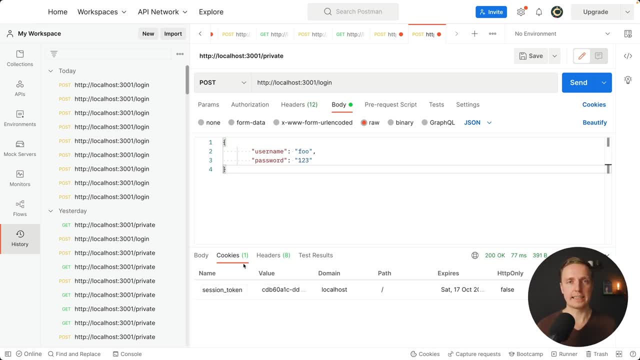 So we add a new value, Which actually means our client should not do anything at all. We successfully got a cookie from our backend, And now every next request of our client will be authorized. This is why now it is time to protect our private route. 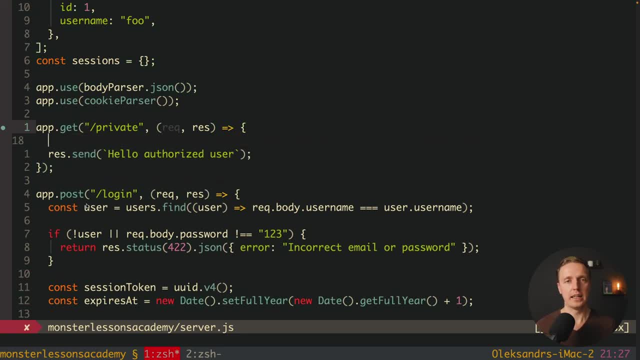 So here we have just res sent, But we want to do a lot of stuff. First of all, we want to try and read our session token, Because only our lockedin user can have this correct session token. This is why here let's read it from our request cookies. 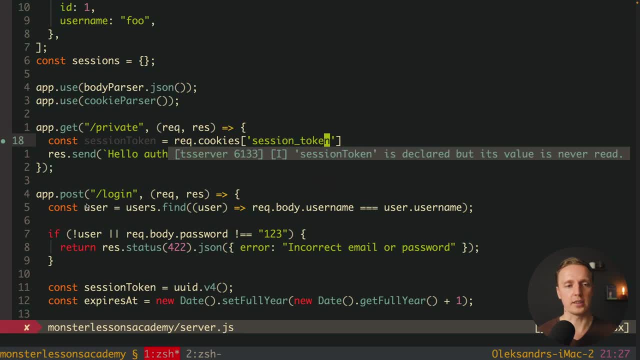 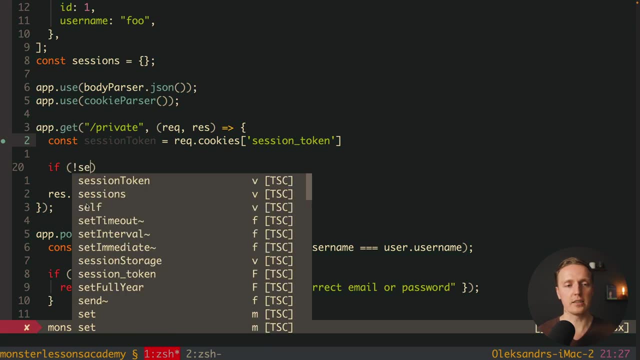 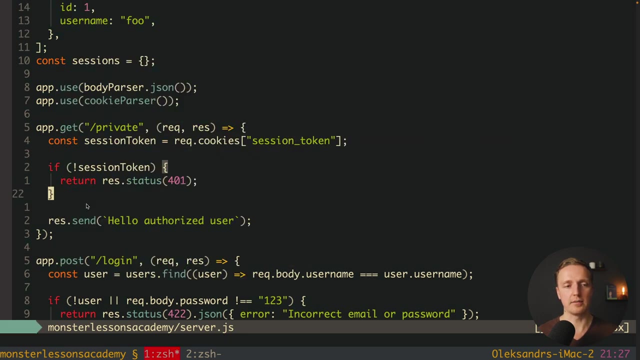 cookies and we are reading here: session underscore token. If for some reason we didn't get a session token, then we just throw for01- unauthorized. So here we can write: ok, if we don't have our session token, then we want to return res status and here: for01.. 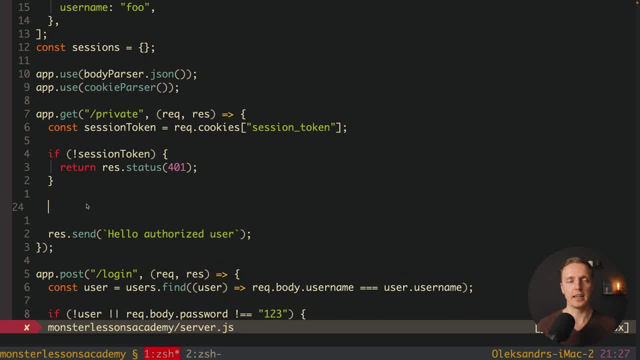 After this we must try to find a session inside the database, Because if we don't have a session, then we are not logged in. This is why here let's try to get current user session, And we are getting it from our session's session token. 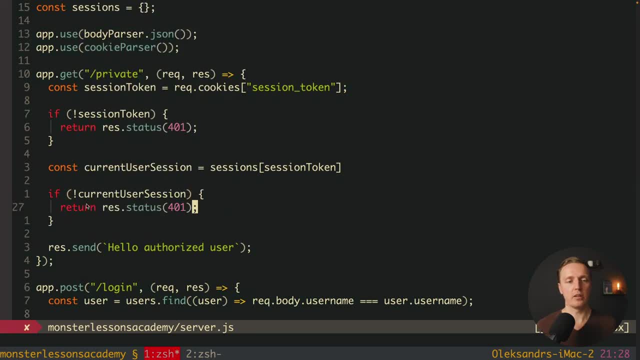 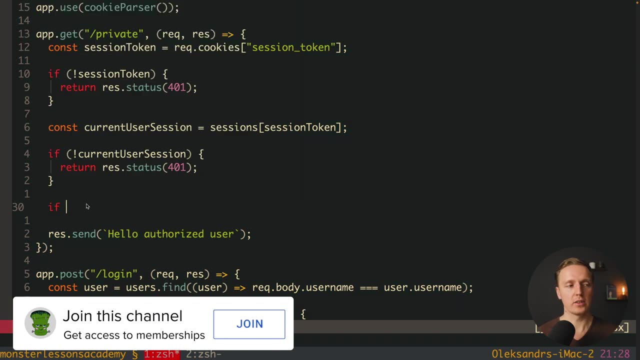 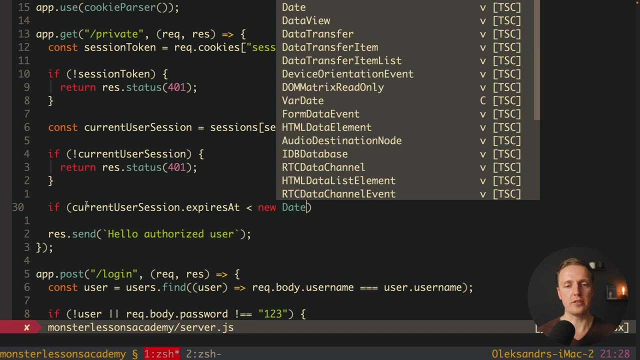 If we didn't find our current user session, then we throw unauthorized again. And the last check that we can do- but it is not mandatory- we can check expiration date. So here we can check that our current user session dot expires at is less than new date. 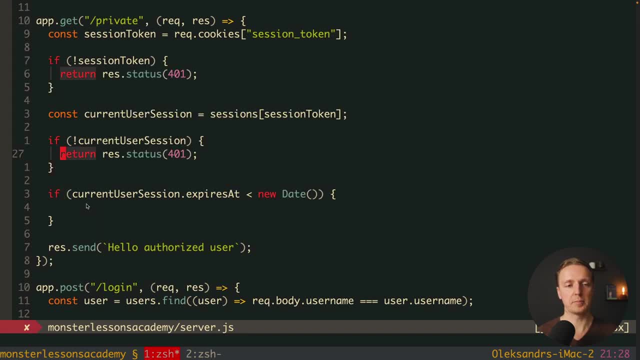 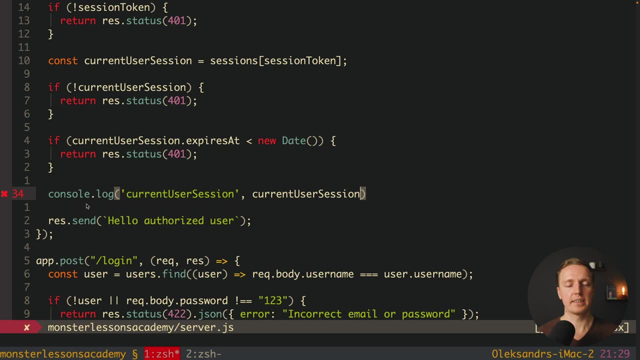 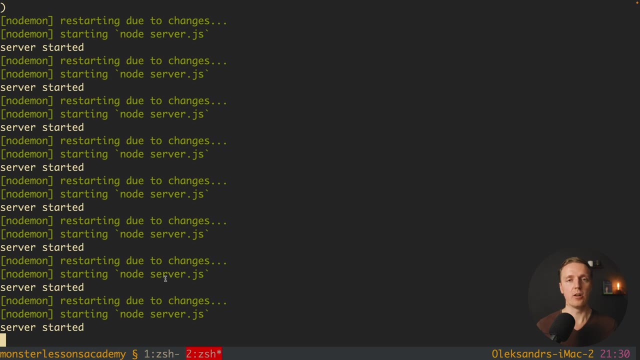 And new date means now, Which actually means it is already expired And we can simply change it. Simply throw here our for01.. Now here I want to console log what we have, and we have here our current user session. It is important to remember that every single time when our server is restarted, all our 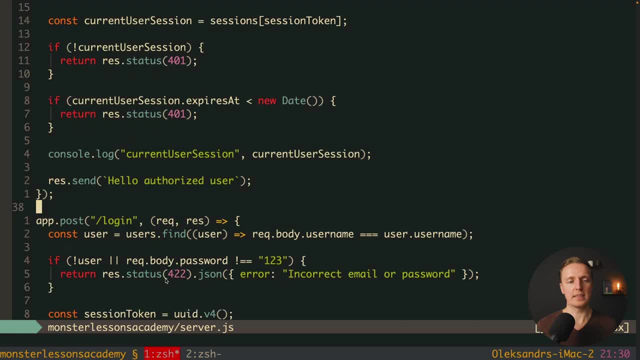 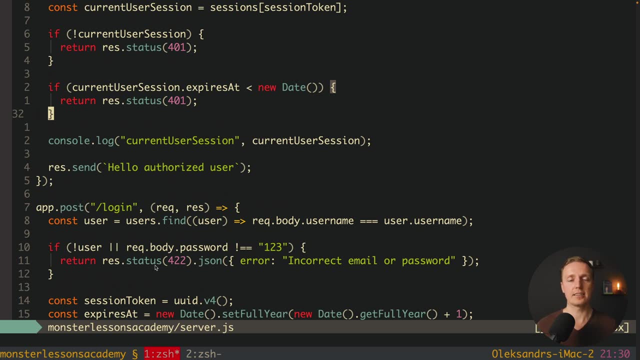 data inside memory are deleted, Which actually means if we are logged in and we created a session, but our server was restarted, then our session is removed. This is not a real database, Which actually means if you are testing this private route, you must first of all make a. 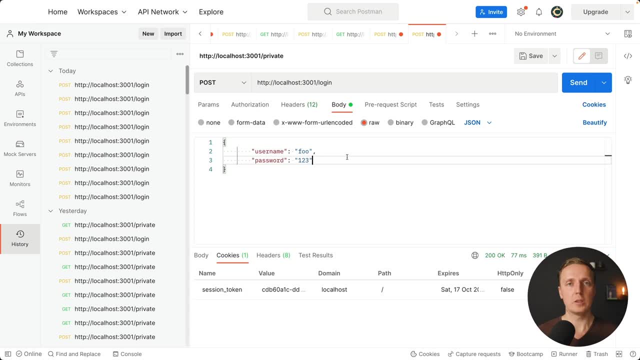 post request after server restart, and then you need to make a request before you will restart your server again. This is why here let's try to login and set the session token, And after this I want to make a get request. And here is our slash: private. 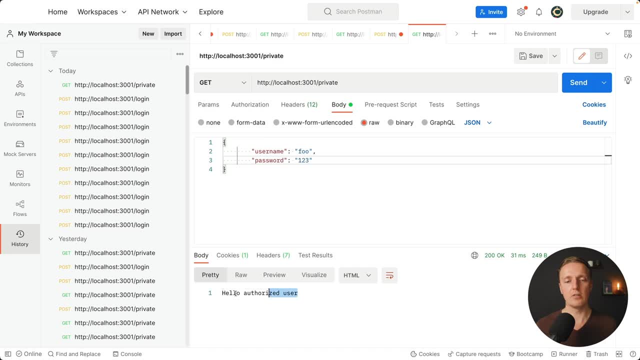 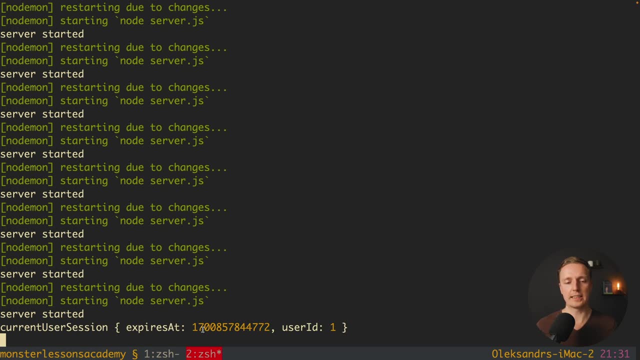 I am hitting here send and, as you can see, here is our body: hello, authorized user. But now inside our console you can see current user session And this is an object with expires at and user id, And now we can directly use our current user session.